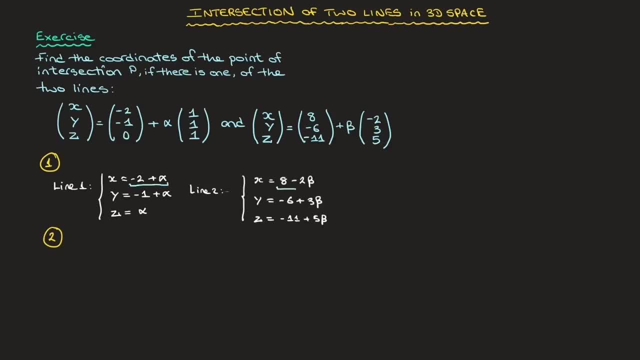 so that would be negative 2 plus alpha equals to 8 minus 2 beta. We'll then do the same for the y-coordinates: that's negative 1 plus alpha will equal to negative 6 plus 3 beta. and finally, we'll do the same for the z, so that will be alpha equals to negative 11 plus 5 beta. 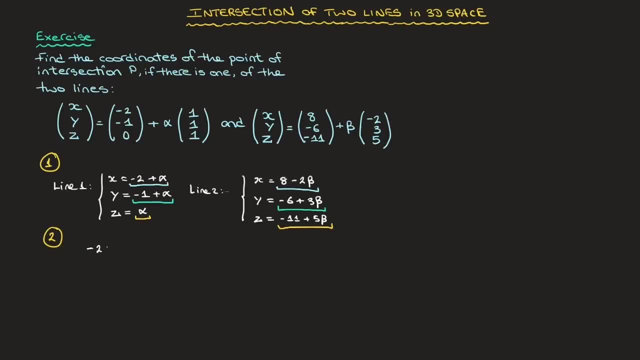 So if I quickly write that, that's our three equations are: negative 2 plus alpha equals to 8, minus 2 beta. negative 1 plus alpha equals to negative 6 plus 3 beta and finally, alpha equals to negative 11 plus 5 beta. 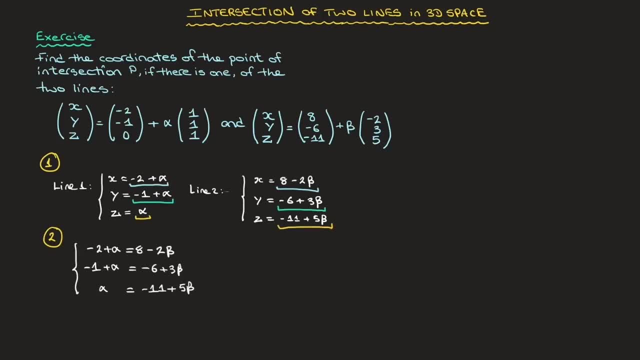 And we can see here that we have three equations with two unknowns. Next, I rewrite these equations, bringing the alpha and beta on the left-hand side and the constant term on the right-hand side of each of these equations, And by all means check, but doing so leads us to alpha. 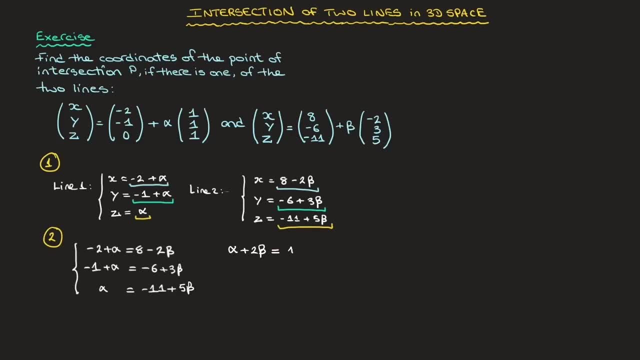 plus 2 beta equals to 10,. alpha minus 3 beta equals to negative 5, and finally, alpha minus 5 beta equals to negative 11.. Done, The next thing we do- so I'll just write 3 here- is use two of these three equations: 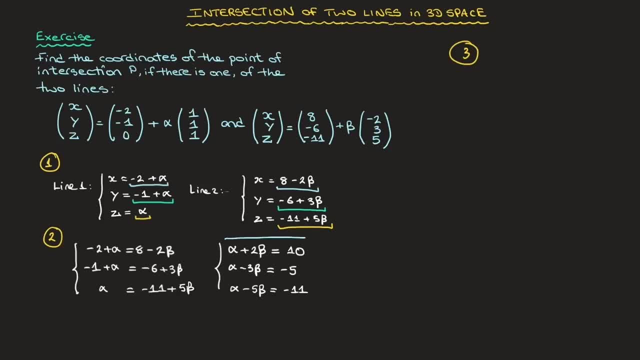 and solve for alpha and beta. So I'll go ahead and use the first two equations that we have here. In other words, I solve the simultaneous equations: alpha plus 2 beta equals to 10, and alpha minus 3 beta equals to negative 5.. 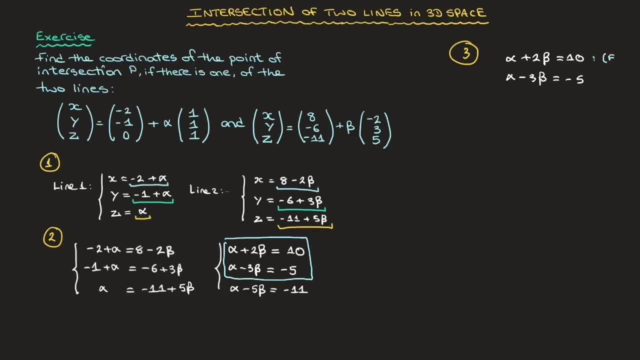 When doing this, I like to name the equations, so I'll call the top one equation 1, and the bottom one we'll call equation 2.. And looking at these two equations, we quickly see that if we subtract equation 2 from equation 1, we'll eliminate the alpha. 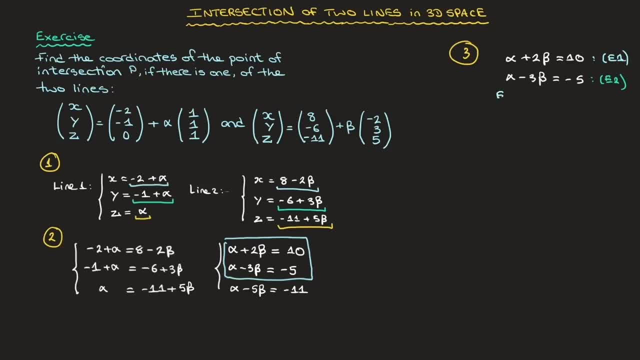 We'll then be able to solve for beta. so let's do that. So I'm doing equation 1 minus equation 2.. So we'll have alpha minus 3 beta equals to negative 5, alpha. so the alphas are gone: 2 beta minus negative 3 beta, which leads to 5 beta. and that 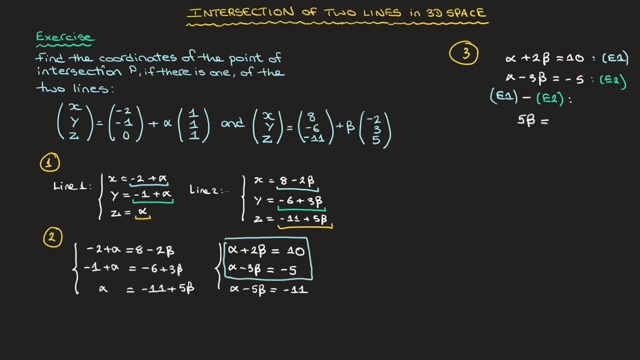 equals to 10 minus negative 5,, which leads to 15.. And we quickly see here that beta equals to 15 divided by 5, which is 3.. Done, we now have a value for beta. We now use this value of beta and plug it. 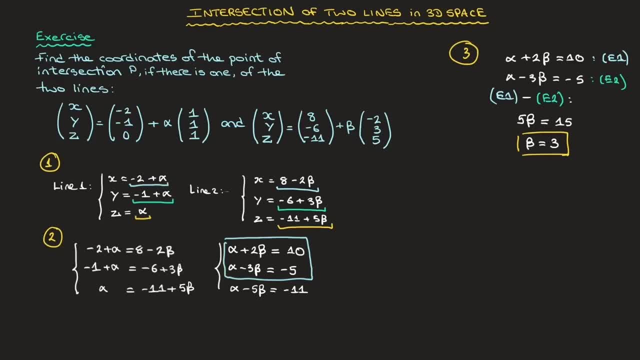 into either of these two equations to calculate alpha. I'll go ahead and use the top equation, E1.. So in E1, replacing beta by 3, that turns into alpha. plus 2 times 3 equals to 10.. That leads to. 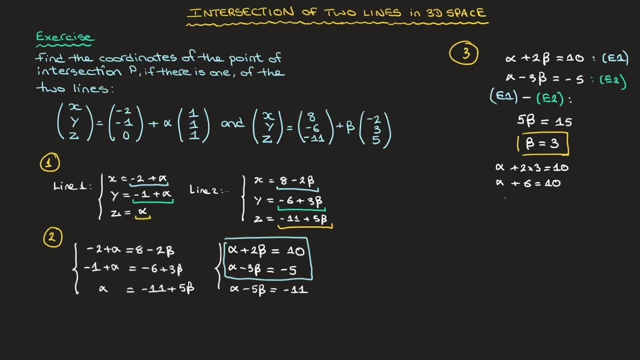 alpha plus 6 equals to 10, and we quickly see that alpha is equal to 4.. Done, And at this stage, we found the values of alpha and beta, for which these lines seem to intersect. But we mustn't stop there. 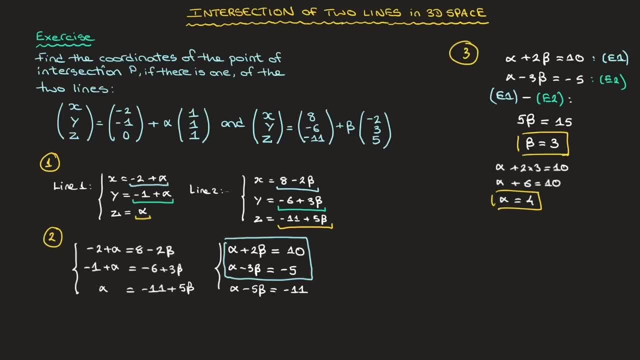 Indeed, when working in three dimensions, the fact that we found a value of alpha and beta for which these lines seem to intersect- we can't stop there. We can't stop there, We can't stop there- does not guarantee that they actually do so, And that's because it's possible that the two lines 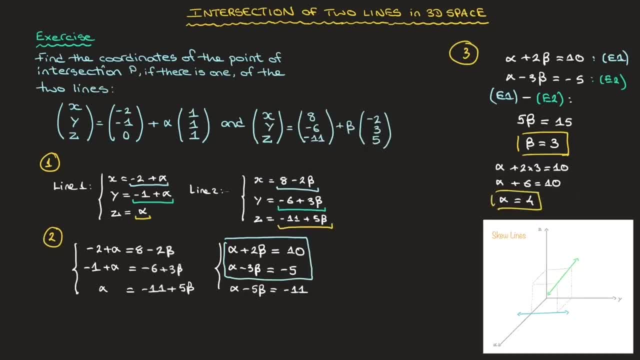 that we have here may be skew lines. Those are two non-parallel lines which are contained in different planes, and so they never actually intersect. And so to determine whether or not these two lines intersect or are skew, we have to go through the next step, step 4.. And in step 4,, 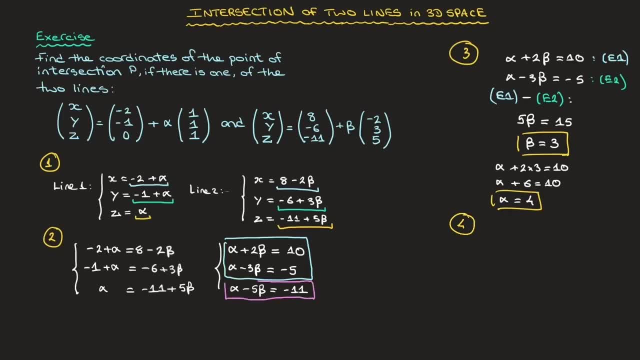 we use the third equation that we have here- the one we didn't use- and check whether or not we replace alpha and beta by the two values, we found it leads to a mathematical inconsistency or not. Here's what I mean: Using this equation here that I've just boxed in pink and replacing 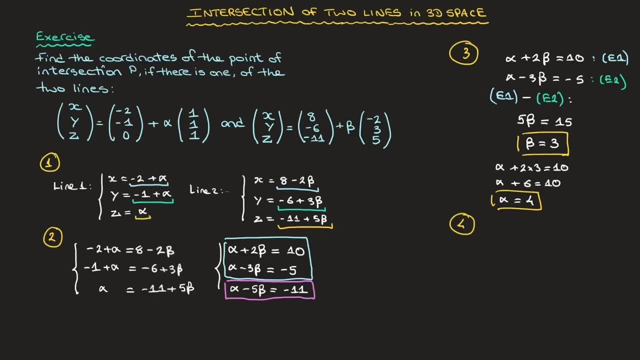 alpha by 4 and beta by 3 leads to 4 minus 5 times 3 equals to negative 11, and that leads to 4 minus 15 equals to negative 11.. Finally, 4 minus 15 is equal to negative 11,. 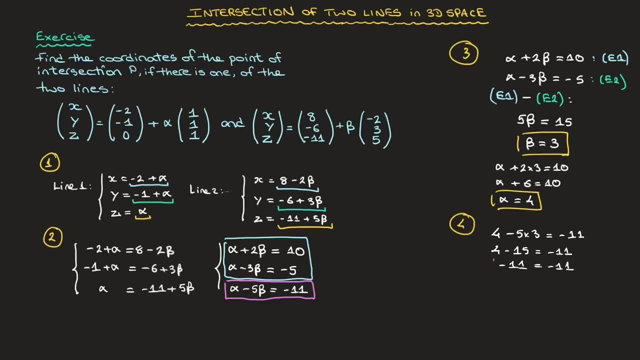 and of course, the right-hand side is still negative 11.. And since the two sides of this equation are equal, we can confirm that the two lines intersect at a point. Had we obtained anything other than negative 11 on the left-hand side here, then that would mean that we're dealing. 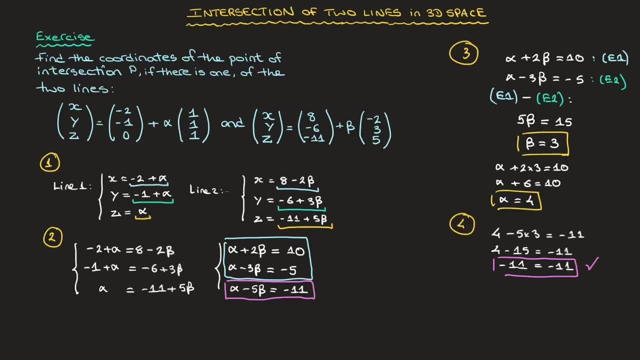 with a mathematical inconsistency, in which case the two lines would be skew lines and would never intersect. Finally, now that we know that these two lines intersect, we calculate the coordinates of the point of intersection, And so I'll just do that here.